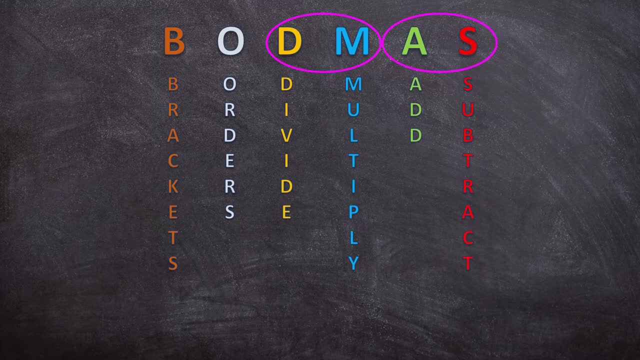 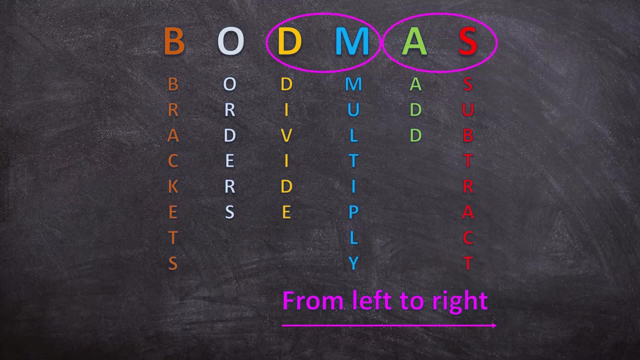 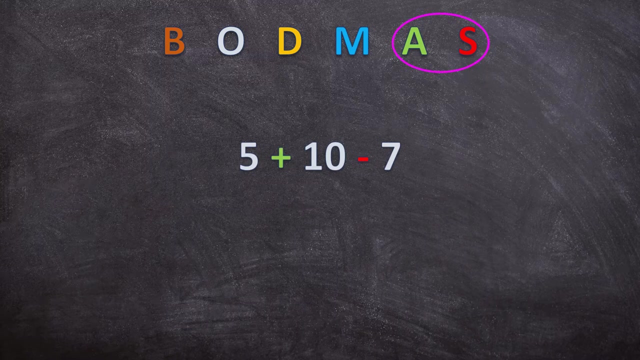 those two. you do it from left to right and the same counts for addition and subtraction. Let's look at the first example. Let's start with an easy example. In this example we only have addition and subtraction, And we know when we have addition. 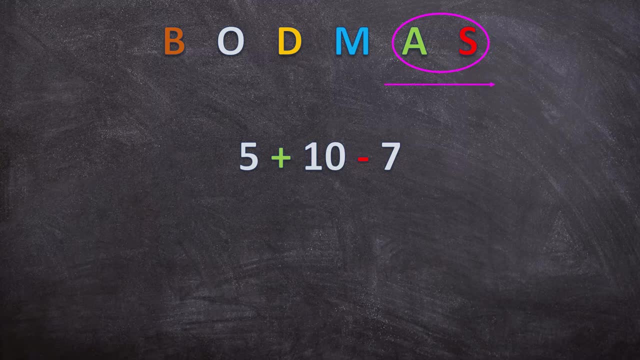 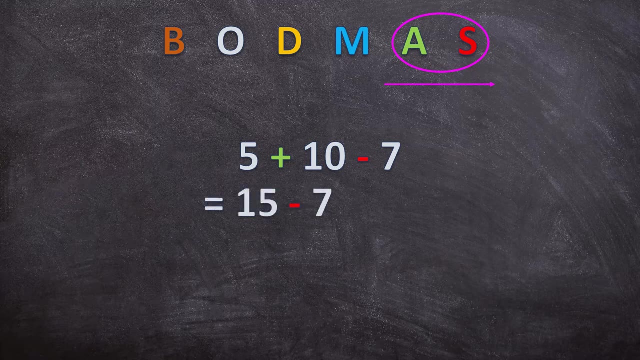 and subtraction together, we go from left to right. So first we're going to add: So 5 plus 10 is 15.. And then we'll subtract: 15 minus 7 is 8.. Now let's look at the next example. 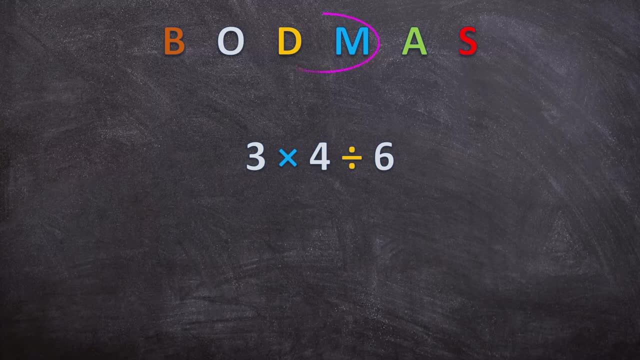 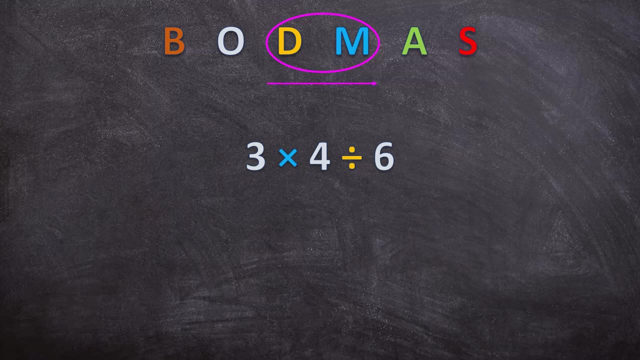 In this example we have multiplication and division, And it doesn't matter in which order they are. We know when we have them both. we go from left to right. So first we'll multiply. 3 times 4 is 12.. 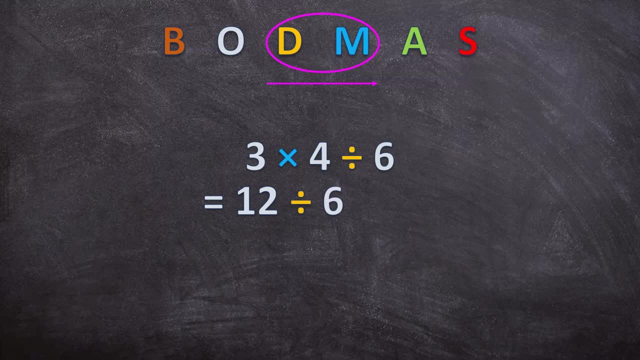 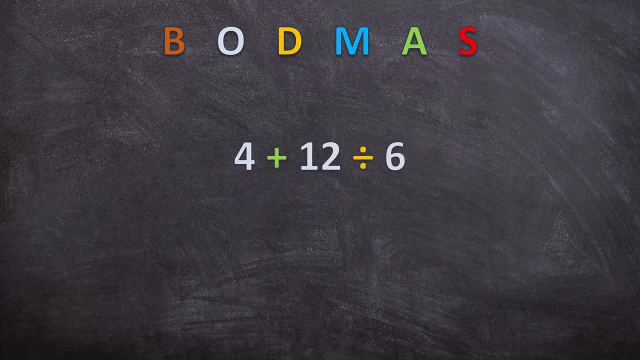 And then we'll divide by 6.. 12 divided by 6 is 2.. Let's look at another example. This one is a bit more advanced. Now we have addition and subtraction, addition and division. when we have division and addition, we'll divide first and then we'll add. 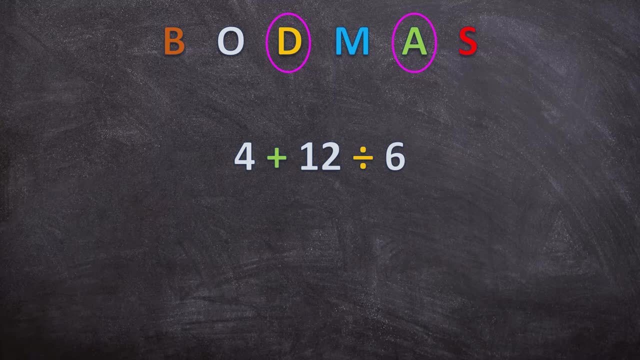 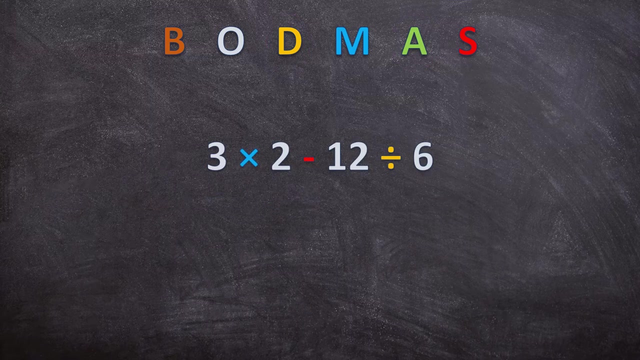 so we're not adding yet. so we just write down the four as it is. we're not touching the four yet, and then we're first dividing. so 12 divided by 6 is 2.. now that we've divided, we can add. 4 plus 2 is 6.. now let's have a look at this example. we have multiplication and division. 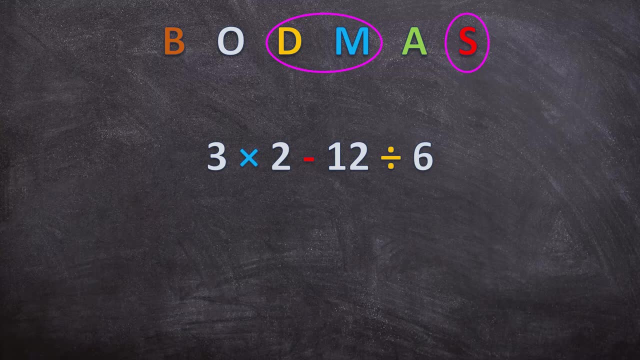 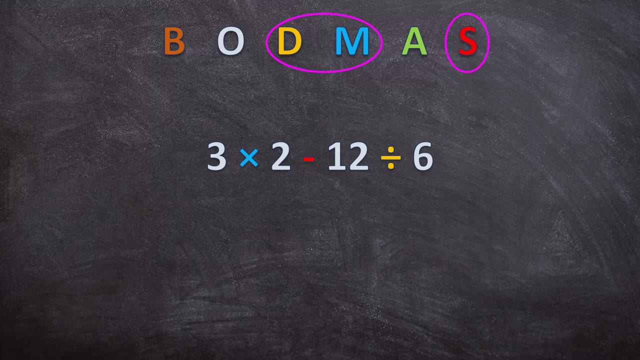 and we have subtraction. so we will divide and multiply first before we subtract. and in which order do we divide and multiply? we start at the left and we go right. so in this case multiply is first. so 3 times 2 is 6.. we don't subtract yet and now we're going to divide. so we write down the. 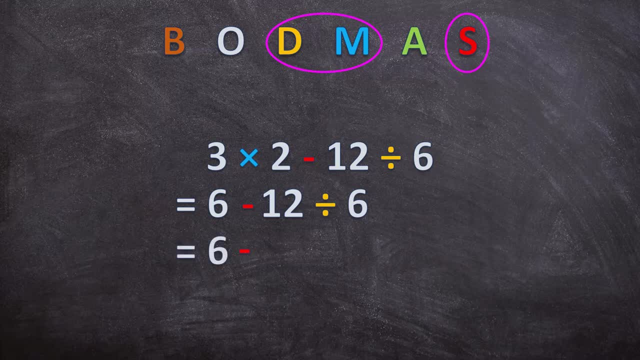 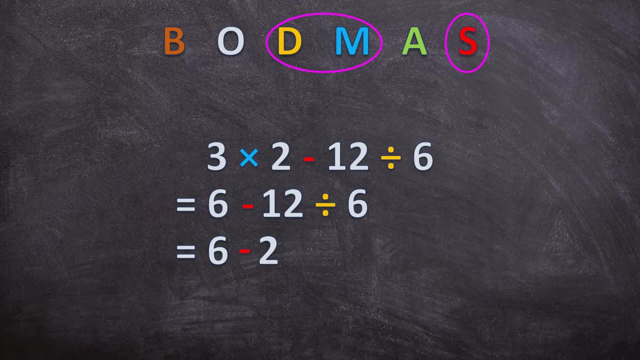 6 and the minus. we're not subtracting yet and we're dividing 12. divided by 6, that will be 2, and now that we've multiplied and we've divided, now we may subtract. so 6 minus 2 is equal to 4.. 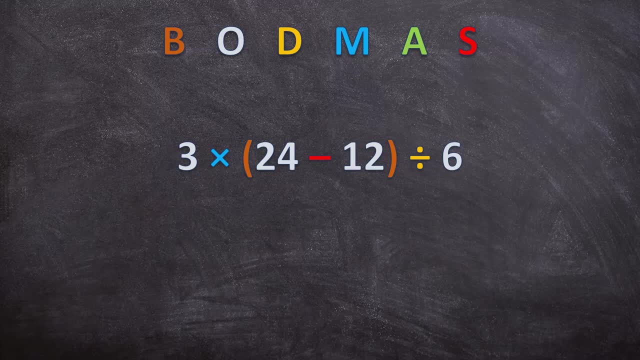 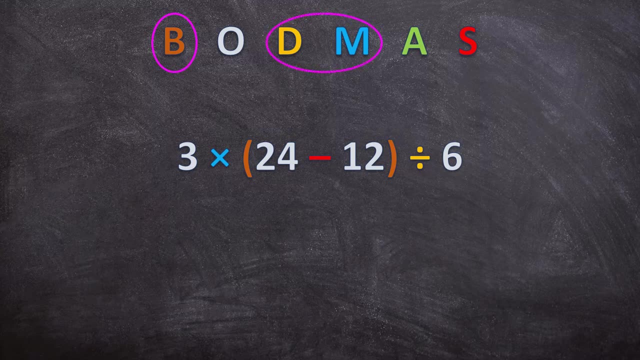 okay, now it's getting more advanced. what will you do here? here we have brackets, we have division and multiplication and we have subtraction. so what's the first thing we're doing? we are doing brackets first, so it doesn't matter that it's a subtraction inside the brackets. 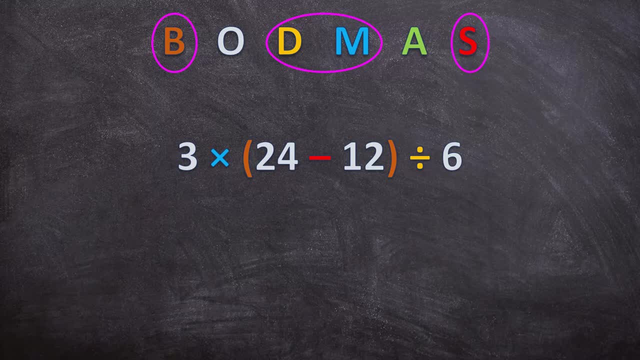 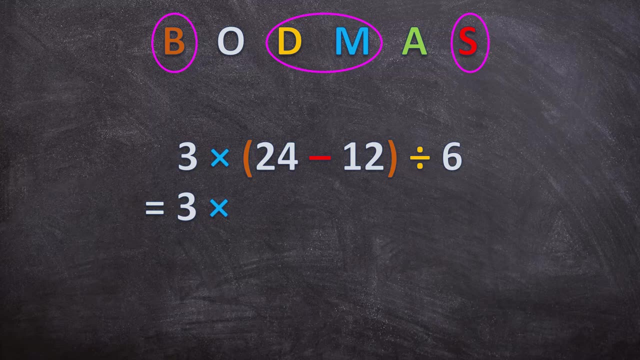 we will do that first, because we do brackets first. so we write down the three times because we're not touching that yet. then we're doing the brackets, so 24 minus 12 is 12, and then we write down the divide by 6.. so now we only have multiplication and division, and we know when. 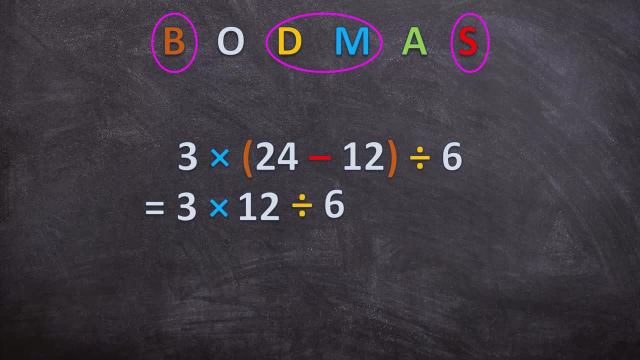 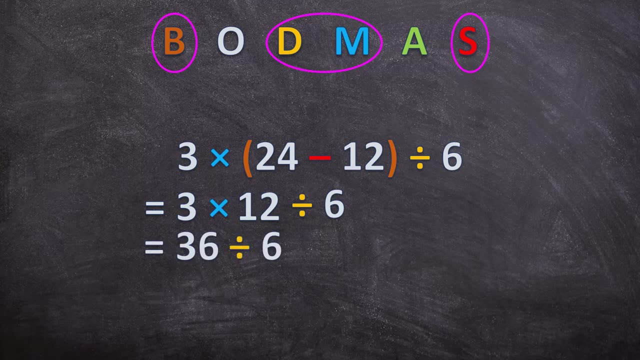 we have them both. we go from left to right. so the first thing we're going to say is: 3 times 2 is 6.. times 12, that is 36. and now we're going to divide by 6, and 36 divided by 6 is 6.. 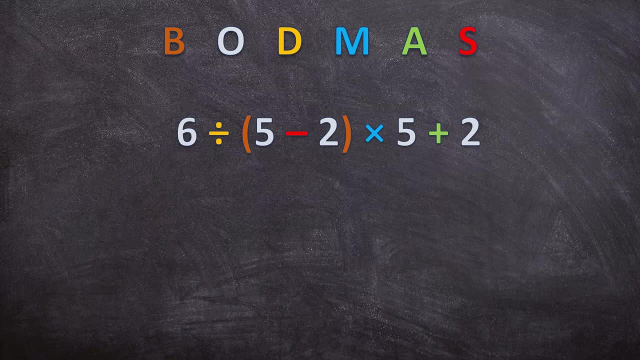 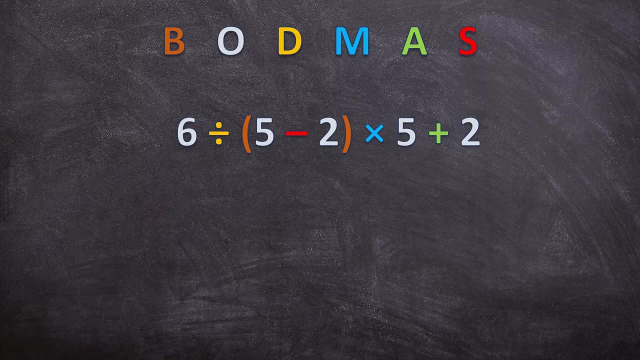 now let's have a look at this one. it seems more intimidating, but if you know your rules, if you know the order of operations and you do it step by step, you will see it's actually really easy. so why do we have here? we have brackets, we have division and multiplication. 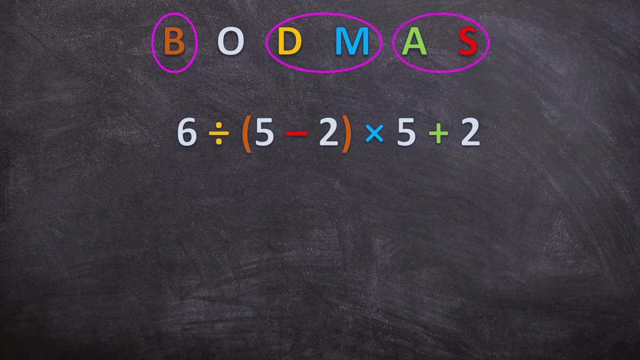 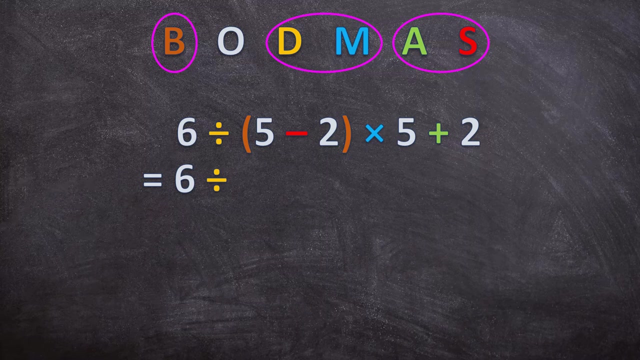 we have addition and subtraction, but what's the first thing? we do? brackets. so we write down the 6 and the divide. we're not touching that yet. now we're doing the brackets. so 5 minus 2 is 3, and then i just write down everything else, because we did the brackets first. now what do we have? we have: 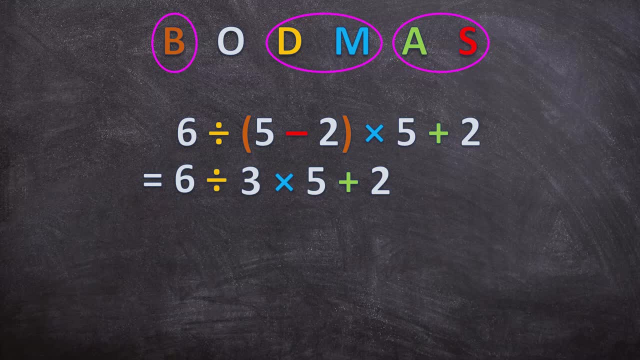 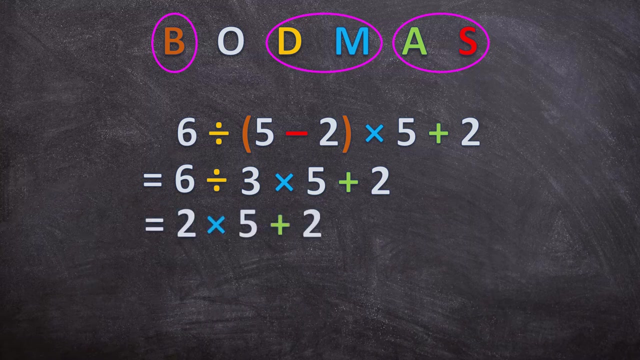 division, multiplication and division and addition. so we know addition will be last, so we'll divide and multiply first, from left to right. so first off we have 6 divided by 3, that is 2, and now we're going to multiply 2 times 5 is 10, and now we're going to add 10 plus 2 is 12.. 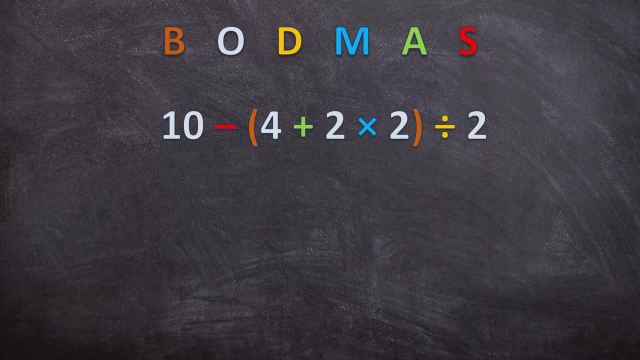 let's have a look at this one now. we have brackets, but we have two operations inside the brackets. but it's not going to bring us down because we know our order of operations. so let's have a look. we have brackets, we have division and multiplication, we have addition and subtraction. 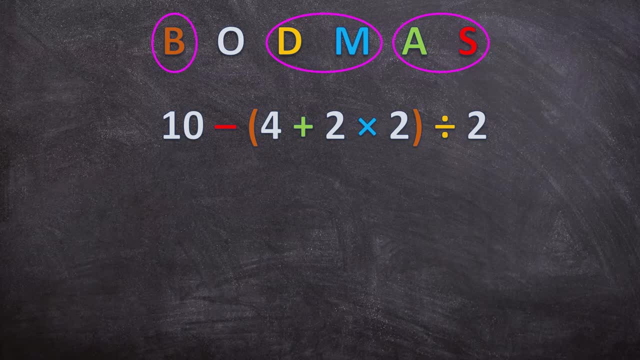 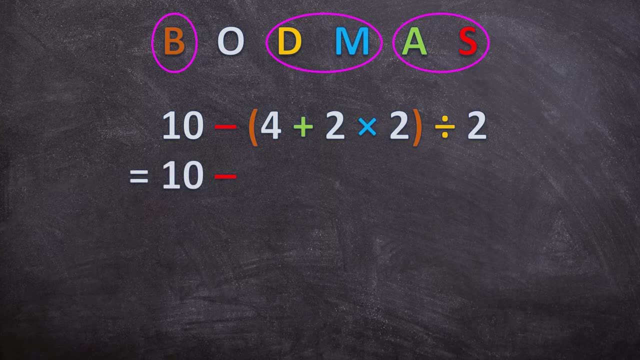 the first thing we do is we write down the 10 minus, because we're not touching that yet we do the brackets first. now, when we look inside the brackets, we have addition and we have multiplication, which one of those are first, yes, the multiplication. so we don't add yet we leave the brackets and we do the multiplication first. so 2 times 2 is 4. 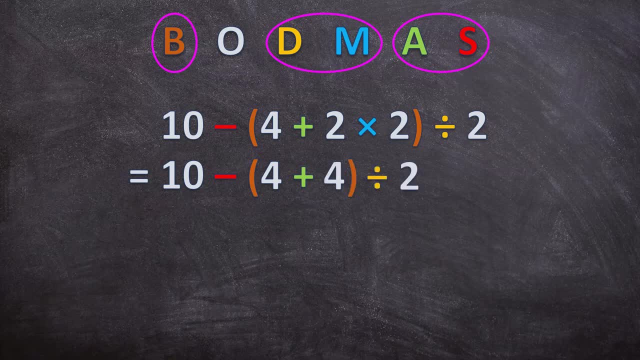 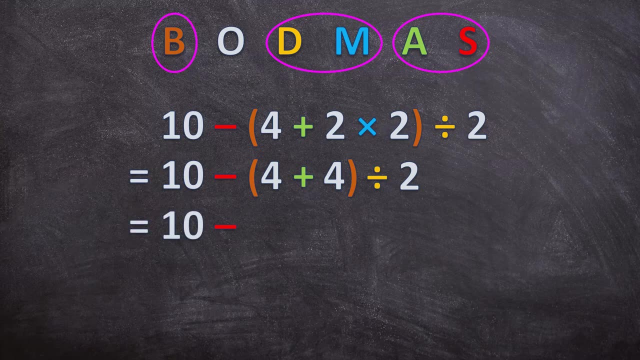 and we close the brackets again and write down the rest of our sum. now let's finish the brackets. we write down the 10 minus because we can't touch that yet. now we're completing the brackets. 4 plus 4 is 8. there's nothing else inside the bracket, so we only add and then we're going to. 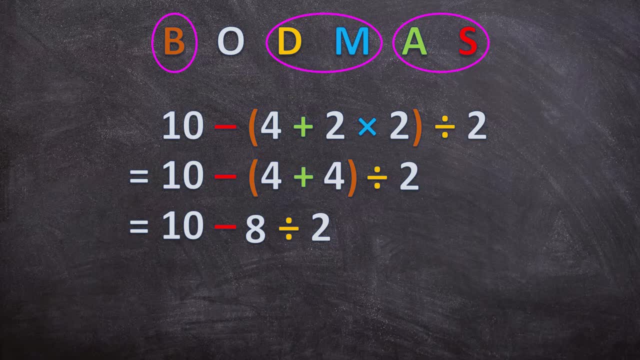 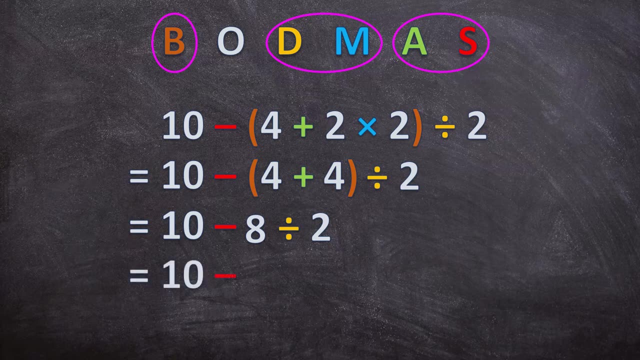 divide by 2. so we've just made this a lot easier. you know that division is before subtraction, so let's do that. we write down 10 minus, because subtraction is last, and we're going to divide. 8 divided by 2 is 4, and now we can subtract. 10 minus 4 is 6.. 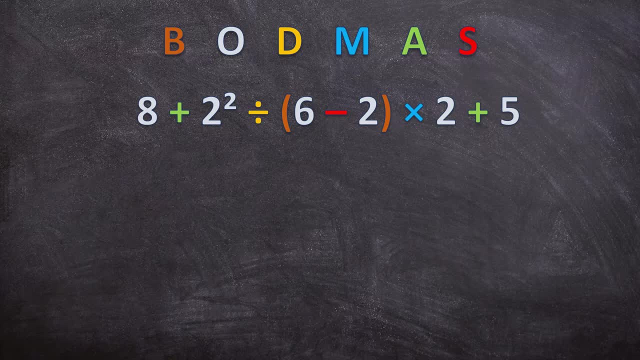 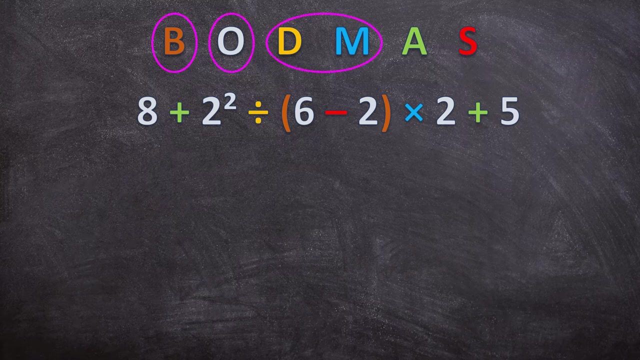 and finally, let's look at this example. we won't let this scare or intimidate us, because we know, step by step, what to do. now. what do we have? we have brackets, we have orders, we have division and multiplication, we have addition and subtraction. so we have all of them. now let's do this step. 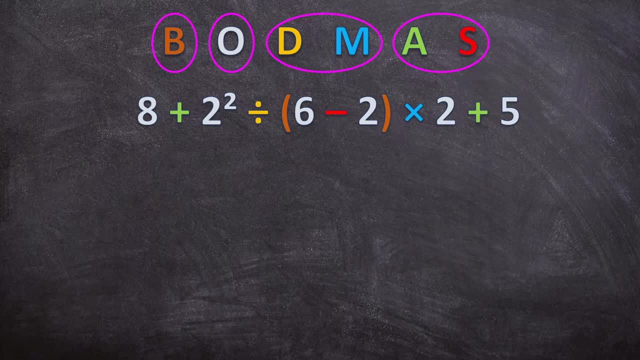 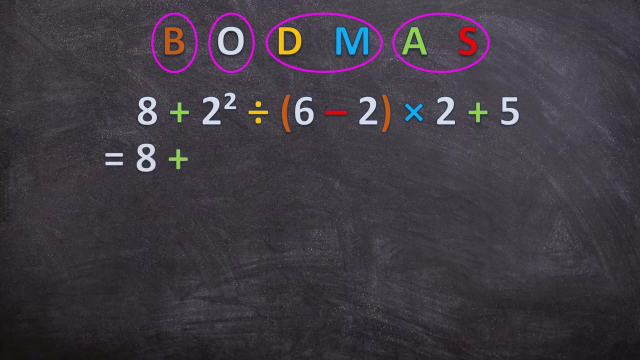 by step and you'll see how easy this is. so the first thing we need to do is take care of the brackets. the first thing we do is brackets. so we write down everything exactly as it is and we only do the brackets. so 8 plus 2 to the power of 2 divide. now we get the answer for the brackets. 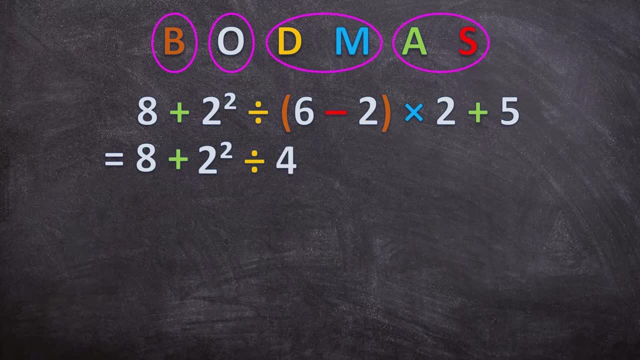 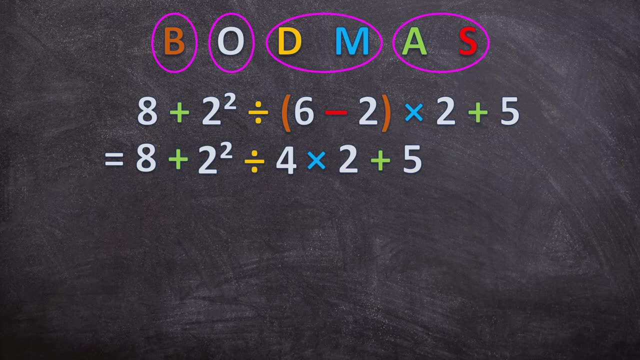 6 minus 2 is 4, and then we copy down the rest times: 2 plus 5. so now we did the brackets, so now we move on to the next thing. the next thing is orders. we have 2 to the power of 2. 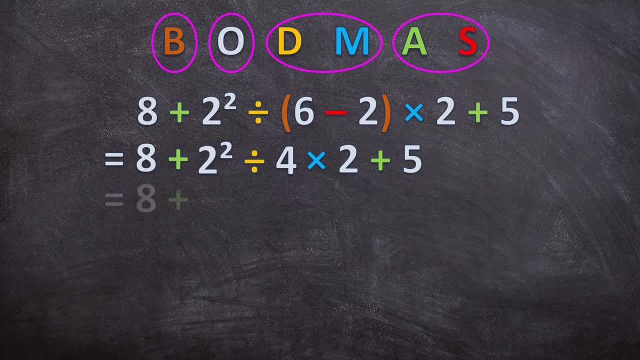 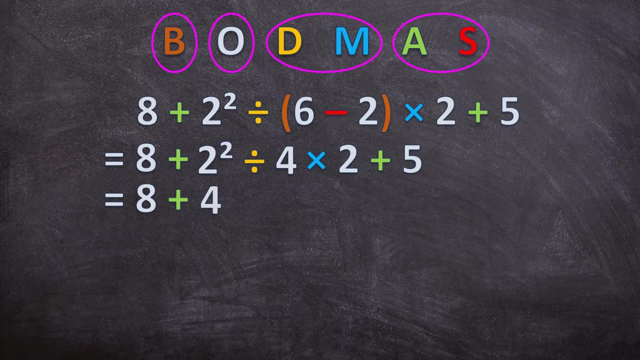 so now we'll do that. so we write down 8 plus what is 2 to the power of 2. 2 times 2 is 4, and then we copy down everything else exactly as it is: divide by 4 times 2 plus 5. it looks difficult in the beginning, but if you do it step by step, 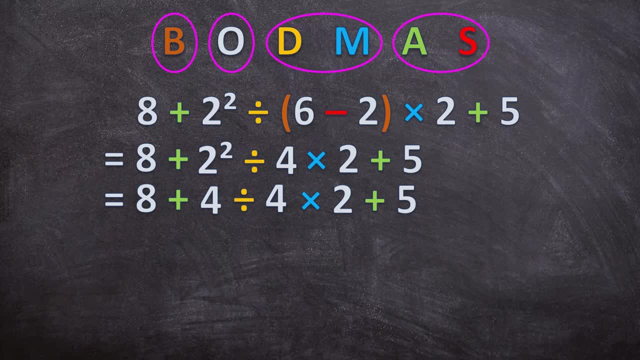 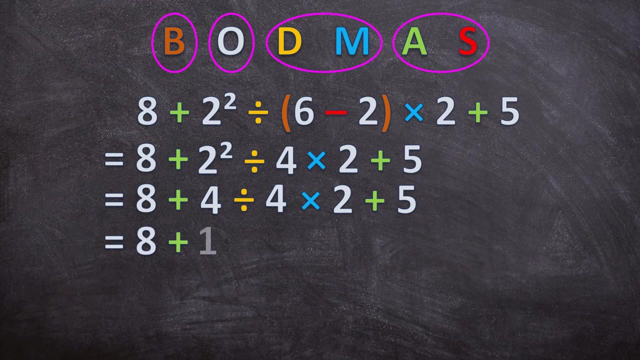 it's actually really simple. now, what do we have? we still have addition, we still have division and multiplication. so what do we do? first, division and multiplication from left to right. so we leave the 8 plus 4, divide by 4 is 1, and then we write on everything. 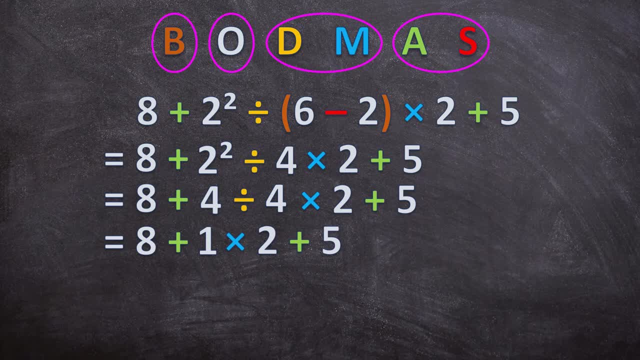 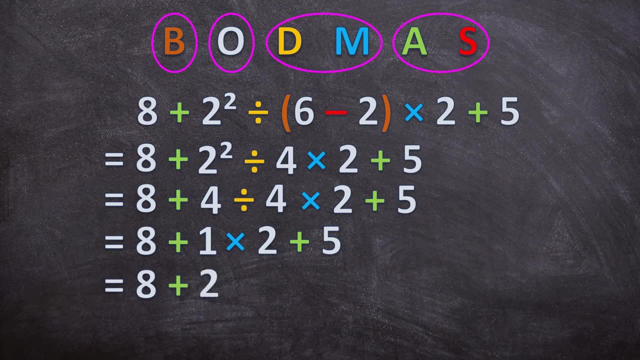 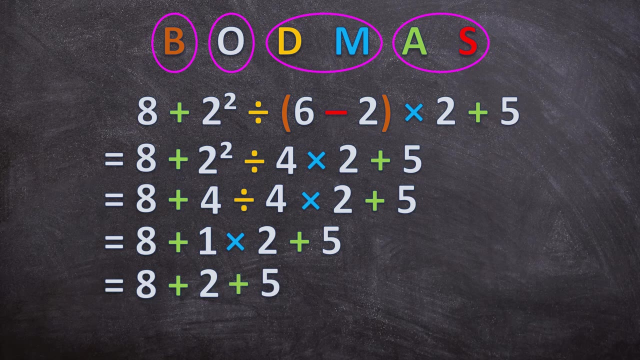 times 2 plus 5. now we're doing the multiplication, so we write down 8 plus 1 times 2 is 2 and we copy down plus 5. so now the only thing we have left is addition. so 8 plus 2 is 10, plus 5 is 4. 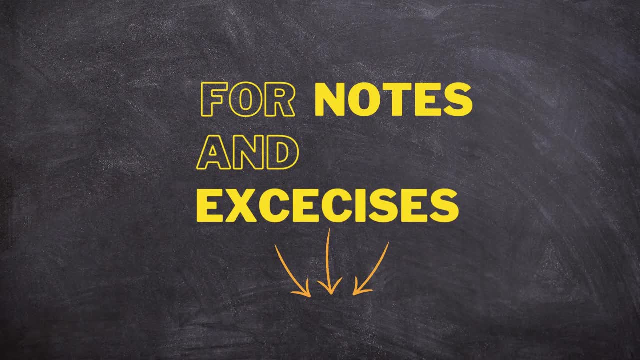 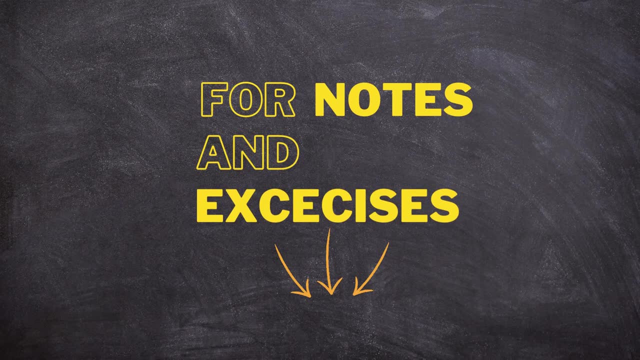 plus 4 is 5, 4, 3, 3, 4, 4, 5, and then we back fingers: เดasty. but you will be surprised how much we have improved over the last couple weeks, contributed to what we can achieve. we really did make it last night, the day before today.